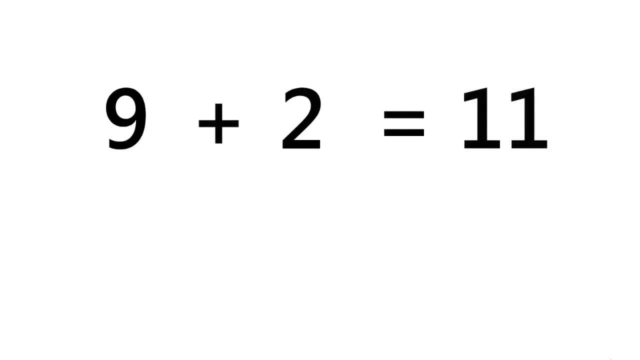 Let's look at adding two single digit numbers. 9 at 2 is equal to 11. 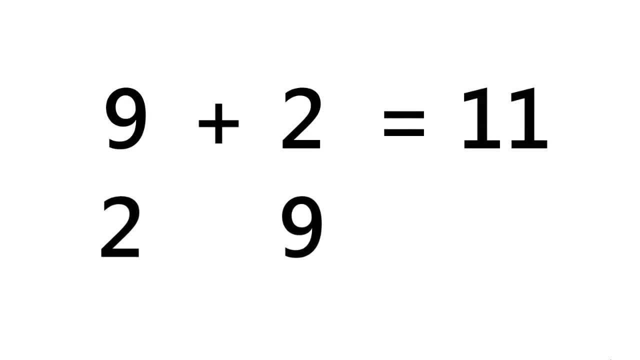 What if we change the order of the numbers to write a new addition problem? According to the commutative property of addition, changing the order of the add-ins does not change the sum. Therefore, the answer is still 11. 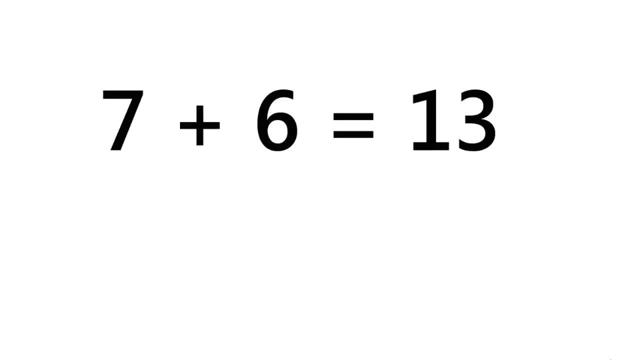 Let's look at another example. 7 at 6 is equal to 13. If we change the order to 6 at 7, the answer is still 13. 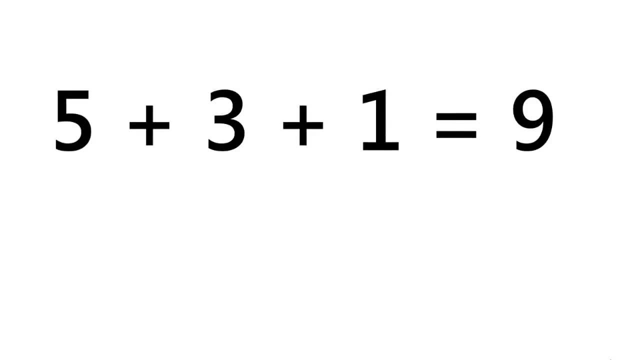 If we group add-ins in an addition problem, the sum will be the same. For example, 5 plus 3 plus 1 equals 9. If we change the equation by grouping the 5 and 3 together, the answer is the same. 5 and 3 gives us 8 plus 1 equals 9. If we change the equation by grouping the 5 and 3 together, the answer is the same. 5 and 3 gives us 8 plus 1 equals 9. 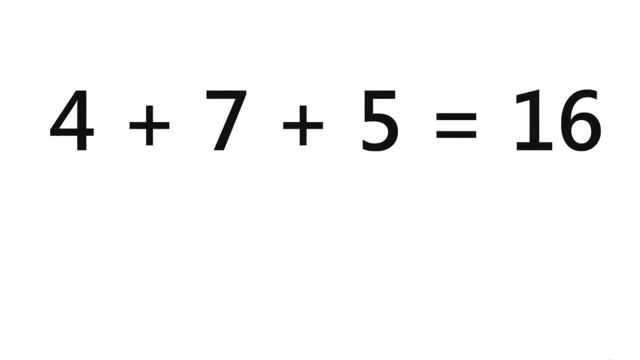 In this equation, we will group the 7 and the 5 together. First, we'll group the 7 and 5 to give us 12. We then add the 4 and 12 for a total sum of 16. 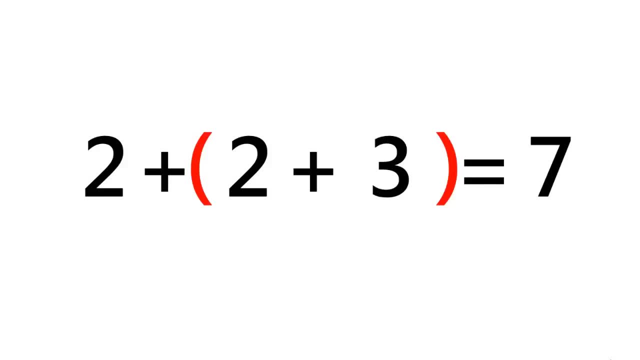 What does grouping look like? Let's look at this equation 2 plus 2 plus 3 equals 7, and think about it in a different way. What if we replaced our numbers with something else? Say, cups of coffee. Instead of grouping 2 and 3, let's group 2 cups of coffee with 3 cups of coffee. 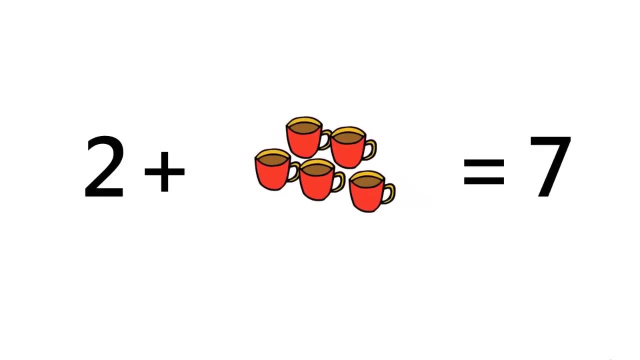 We now have 5 cups of coffee grouped together. Let's replace our remaining number 2 with 2 cups of coffee as well. We can now see that 2 cups of coffee add 5 cups of coffee gives us a total of 7 cups of coffee. 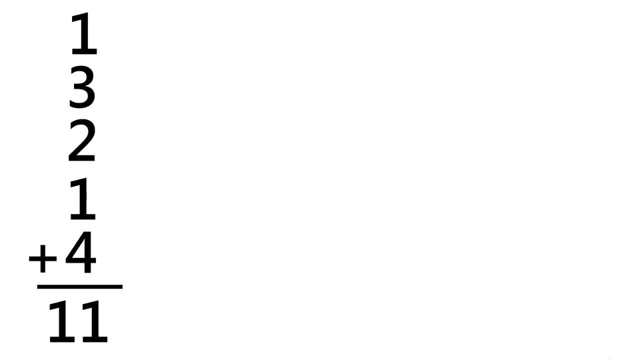 To make it easier to add more than two single digit numbers together, we can work our way down through this problem. Let's add the first two numbers together. 1 add 3 is 4. Now we move the 4 down and add it to the 2, which gives us 6. Moving the 6 down and adding it to the 1, we get 7.